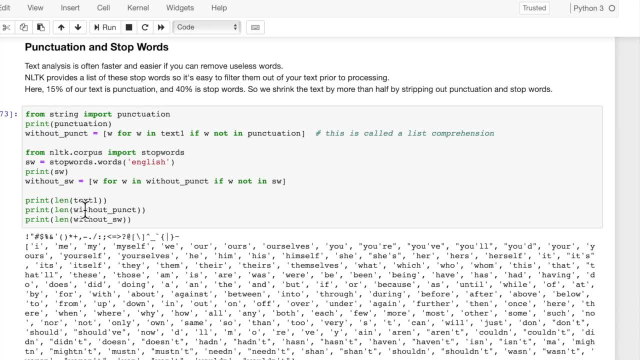 Let's go to the stop word list now. So I print the length of text before we took out anything. Then I print the length of text without the punctuation and then without the stop words, And you can see that we started out with a 260,000 word text which, without the punctuation, 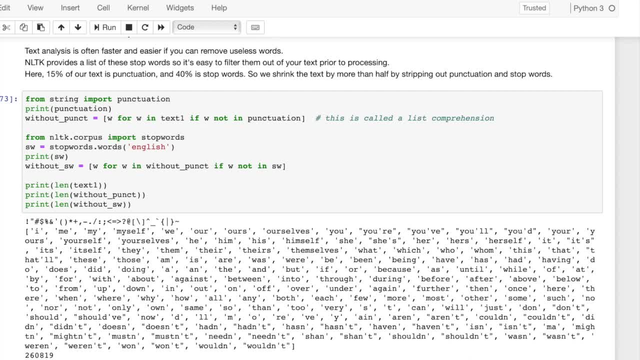 got down to 221,000. And then, when we took the stop words out, it got down to 122,000.. So we reduced the size of our text by about 60% by stripping out all of the useless words and punctuation. 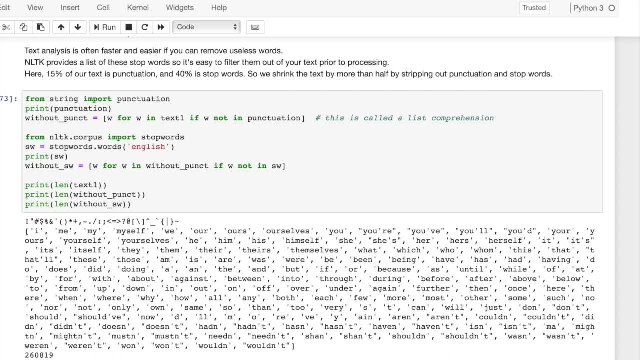 Now we have a much smaller document to deal with, so we can analyze it much more quickly. And you'll see that, as you have a very large corpus, or a very large document that you're analyzing, some of these algorithms are going to run really slowly. 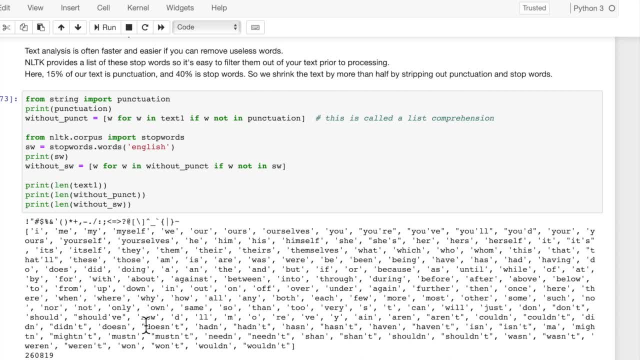 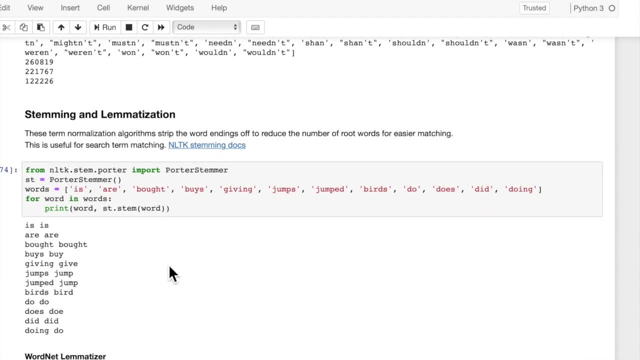 So you want to chop out as much useless stuff as you can. that's going to speed up the run speed of your algorithms. So next, stemming and limitization. So this has some specific uses. It's especially useful, I think, for search engines, because you have a lot of different forms of words. 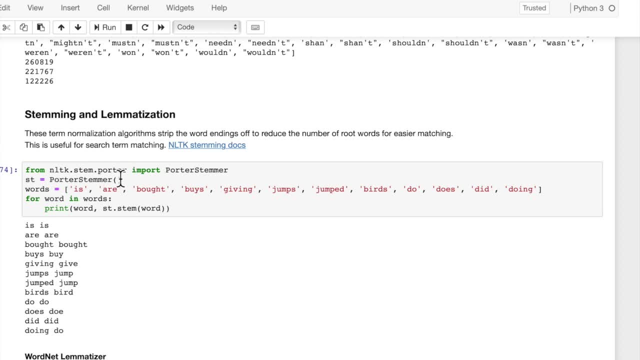 So let's see how this works. First, we're going to use the Porter Stemmer. There are several different stemmers that you can play with. I think there's a Stanford one. Anyway, I put a link to the documentation here. You can look at the stemming docs and you can try out different ones. 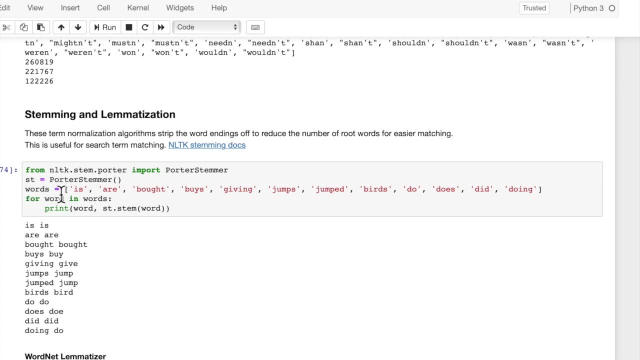 The Porter Stemmer is a really good one that I've used before, And here I'm just going to create a list of words. is are bought, buys, And what we want to see is how it normalizes. It normalizes these words. 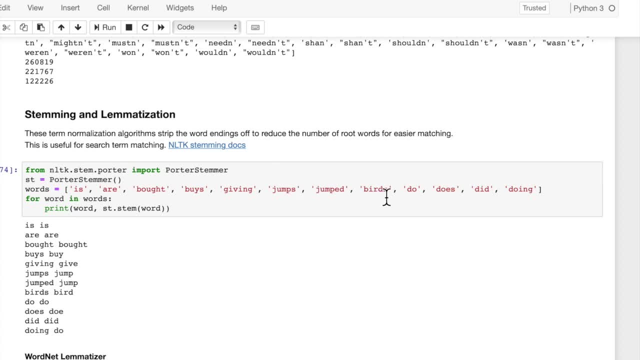 It normalizes them by basically stripping off plural forms of the verb or past or present tense of the verb, and tries to give you a single word instead of five different forms of a word. So for each one of those we're going to print out the word and then the stemmed version. 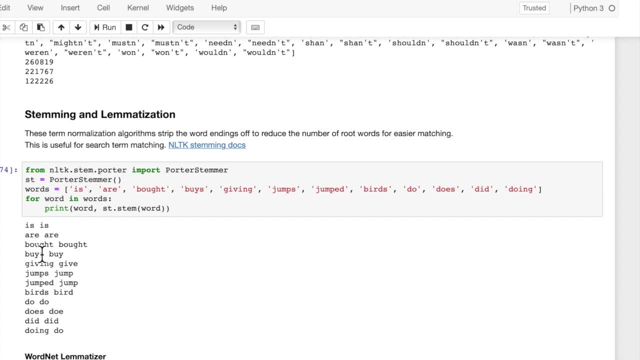 of the word. So is doesn't change Are doesn't change. Bought doesn't change Buys. it just strips off the S Giving, it strips off the ING and puts an E on the end, So it gives us the. 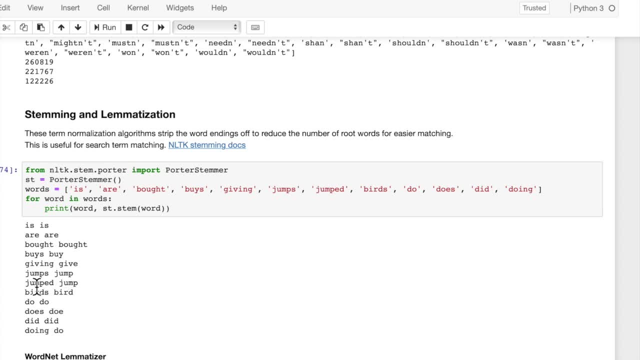 Present tense, the verb Jumps again And you can see how it's normalizing a lot of these words- Not all of them. Look some of them. it converts it to not a word, D-O-E instead of does. 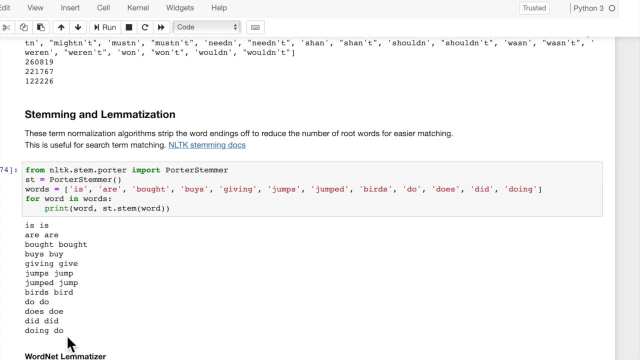 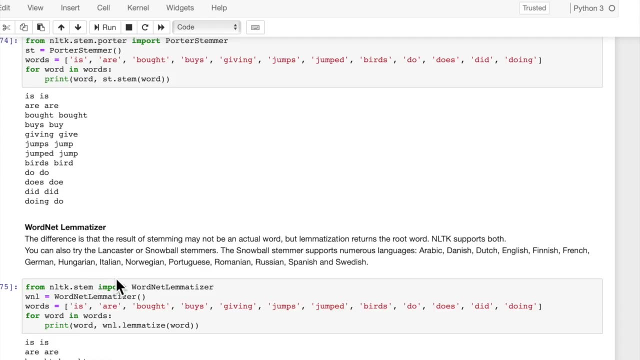 So that's one of the issues with stemming- is that the result you get may or may not be an actual word. Maybe that doesn't matter And the lemmatizer does something very similar, except in theory. it always gives you a word back. 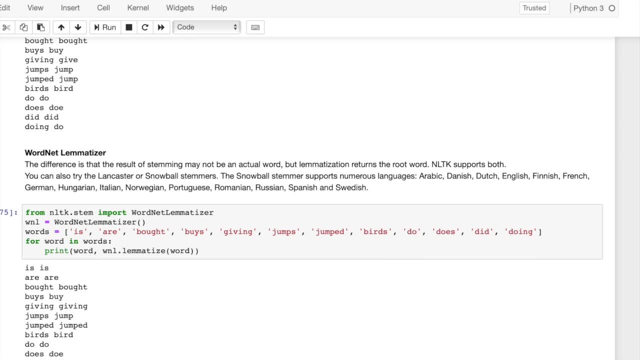 So you'll see down here, though for does it still gives you doe back D-O-E, And most of the answers are basically the same. I think the stemmer does a better job than the lemmatizer, but you can try them both. 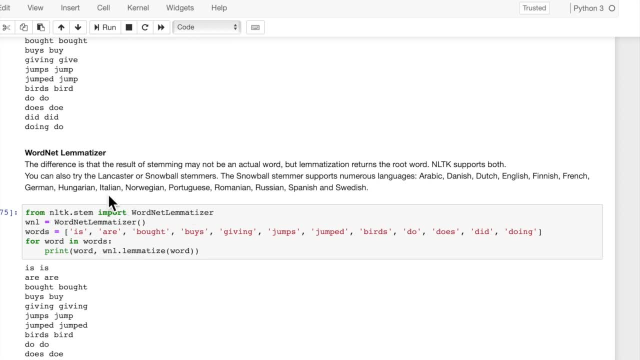 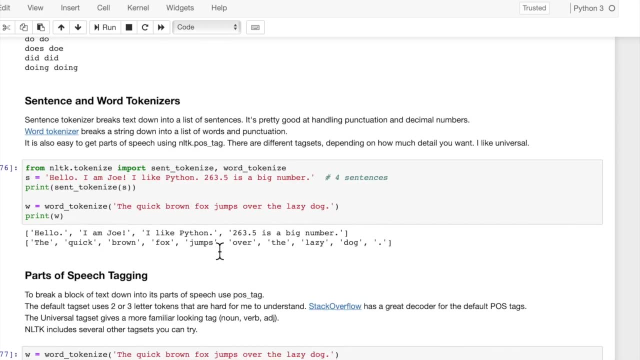 out if you want. Also, the lemmatizer has multiple languages. There's a bunch of different languages that you can try out. The snowball stemmer supports all these different languages, So let's look at sentence and word tokenizers. 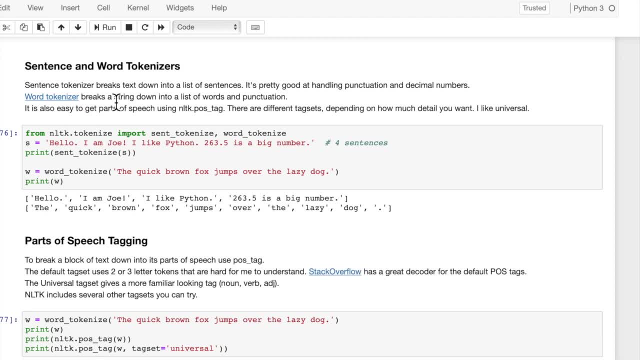 So when you're given a block of code, A block of text, maybe an entire document or a sentence that is in text format, it's just a long string, And what we want to do is break that down to a list, And that is what a tokenizer does. 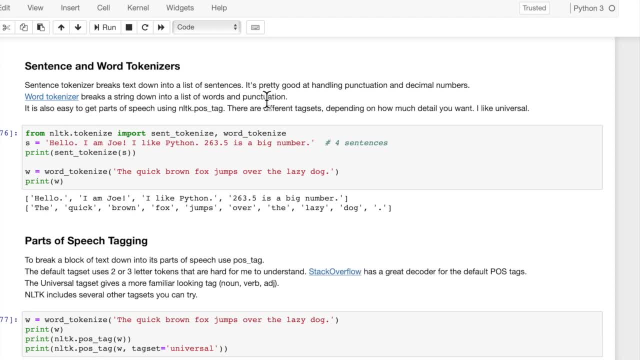 It breaks this string down into lists and it determines where the breakpoints are. And that sounds easy, but it's actually a little hard to do sometimes. So the tokenizer does a really good job with that. So we'll do NLTKtokenize- import- sentTokenize. 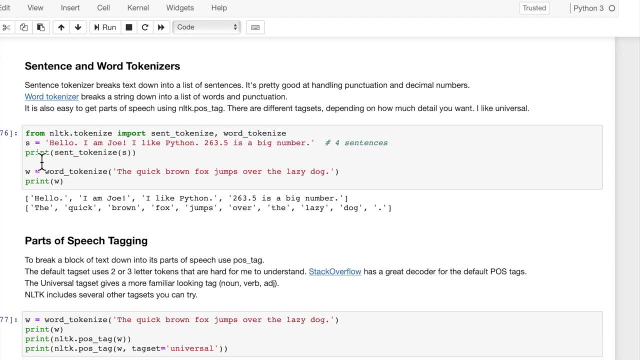 And WordTokenize. We're going to use those two libraries. So hello, I am Joe. I like Python. 263.5 is a big number. Now, this is a little bit tricky. This is actually four sentences. Hello is a sentence in itself. 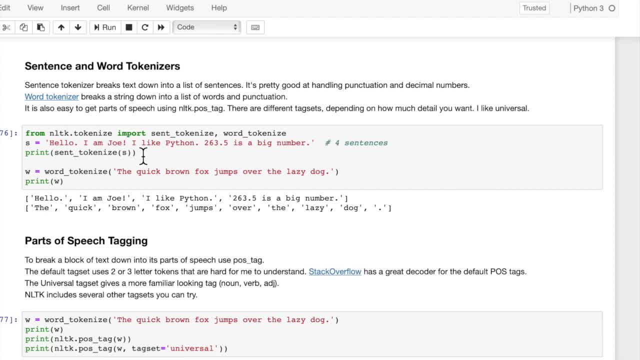 I am. Joe has an exclamation point instead of a period at the end. I like Python is a pretty straightforward sentence. But gee, look, this sentence starts with a number instead of a capital letter And it has a decimal. The decimal plays right in the middle of the number. 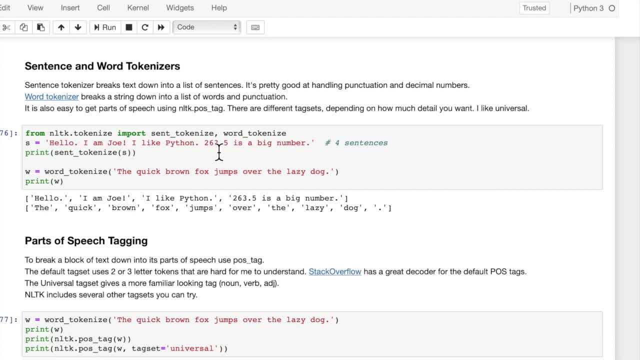 So that could trick our tokenizer. But what happens is it doesn't trick the tokenizer. You can see that the tokenizer we do a sentence tokenization here And the sentence tokenizer gives us back four sentences. So it's pretty smart. It's pretty hard to fool the sentence tokenizer. 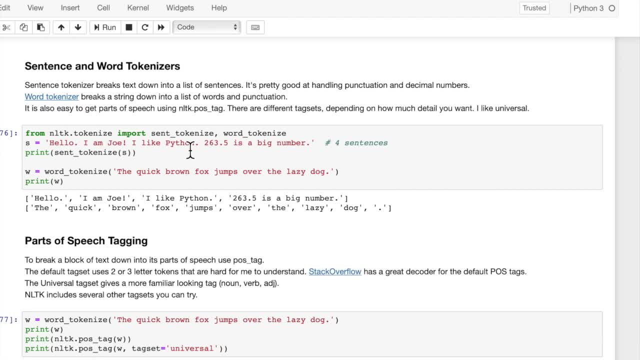 It does a nice job of breaking your text down into sentences. And then the WordTokenizer. we just picked a text string here and it breaks down the entire text string into lists, Into tokens, and it puts them into a list. So you can use the trick we showed up above, using the list comprehension to get rid of 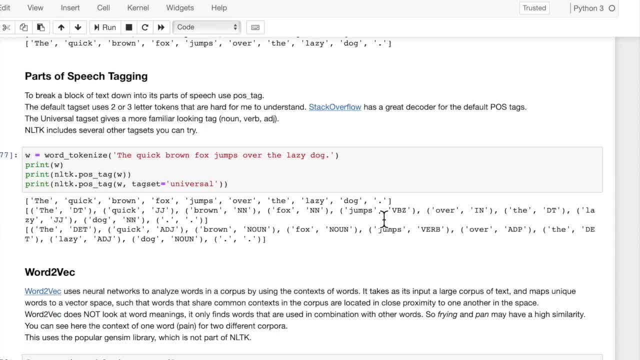 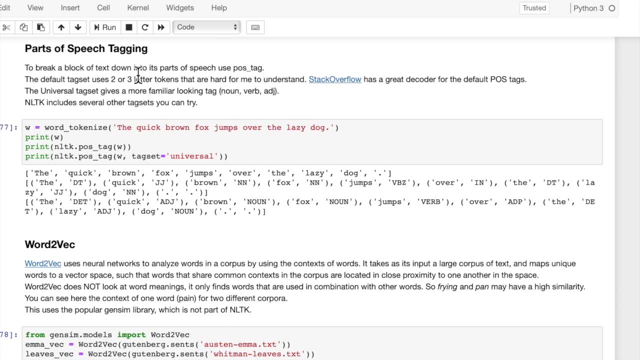 the punctuation, if you want. Next we'll look at parts of speech: tagging- Sometimes this is just called tagging And it's abbreviated a lot of times POS, So to break the text down into its parts of speech like noun, pronoun, verb, adjective. 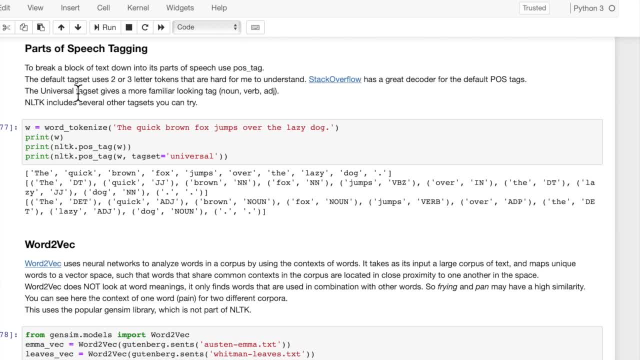 whatever You want to identify those parts of speech, sometimes That's an important part of natural language processing. So we have a sentence: the quick brown fox jumps over the lazy dog, which, by the way, is cool because it uses up every single letter in the alphabet. 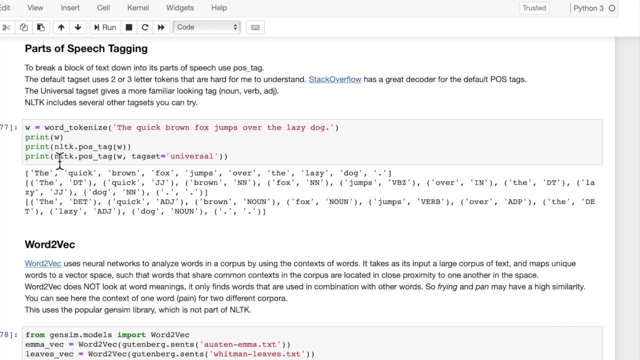 Anyway, we print that sentence and then we identify the parts of speech tagging with the default tag set, So we just pass in W as an argument And what we get back is: gee, what the heck is DT? I don't know. 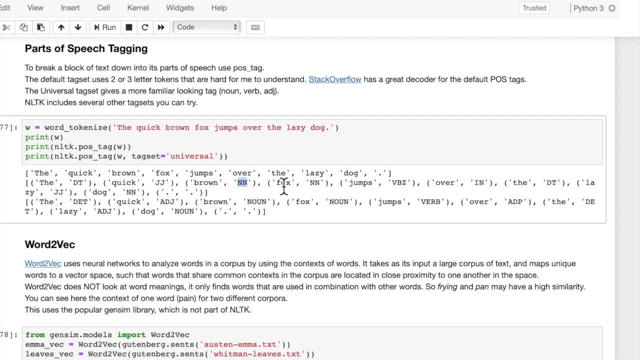 What is JJ? Yeah, I don't know. So these are kind of codes for different parts of speech And they're not very obvious to me. So you can use that if you want. But what I like better is the universal tag set, because it's a little more descriptive. 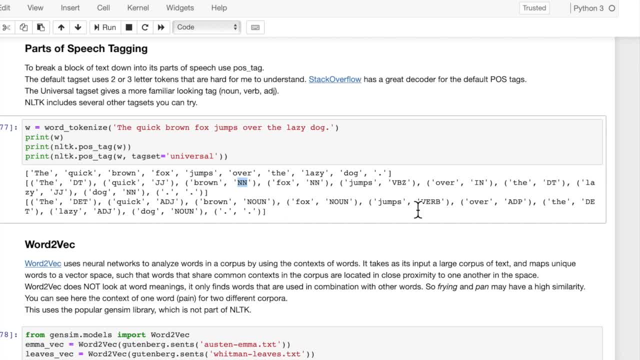 It gives you ADJ for adjective or noun for noun, verb for verb and so on. There are a bunch of different tag sets in this library, So you can try different tag sets if you want.